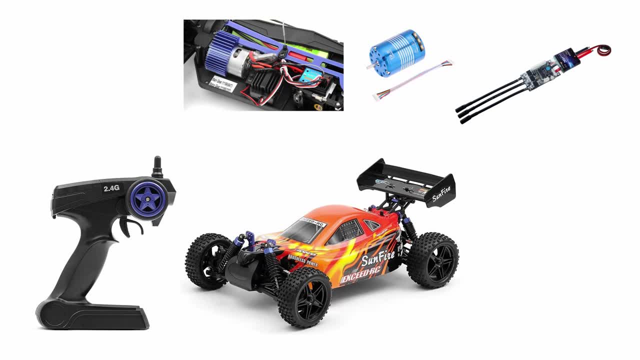 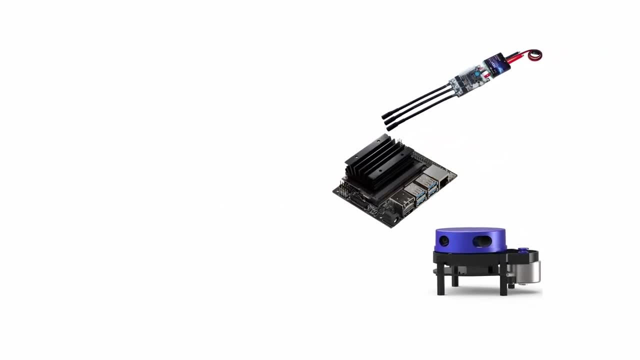 I will explain later why did I choose these components. but I also bought a lidar from ID Lidar and a Jetson Nano, which is the embedded computer. Let me go quickly to each one of these components to get a micro vision of the system. 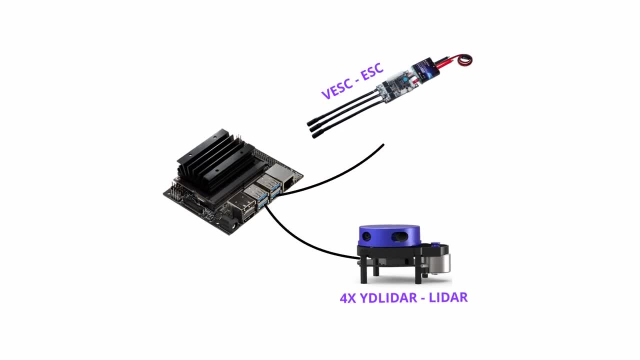 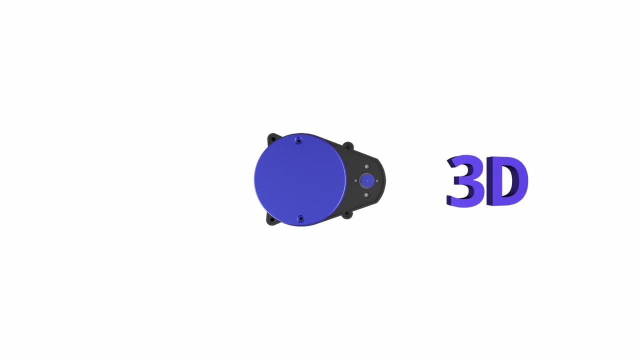 Our main board is the Jetson Nano. Connected to it we have the lidar and the VASC. The lidar is just like your eyes, but instead of seeing color, it sees distance in 3 or 2 dimensions. In my case, since the budget is limited, I got a 2 dimensions lidar. 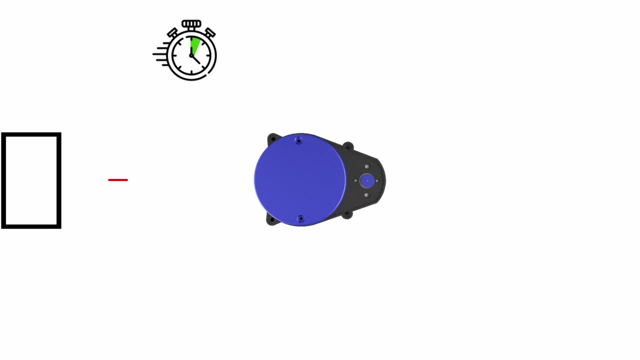 They work by measuring the time that takes to a beam of light to go out of the laser and come back to the sensor. Since we know the speed of light, we can estimate the distance. To create a 2 dimensions, low cost lidar. most companies put a sensor on the base. 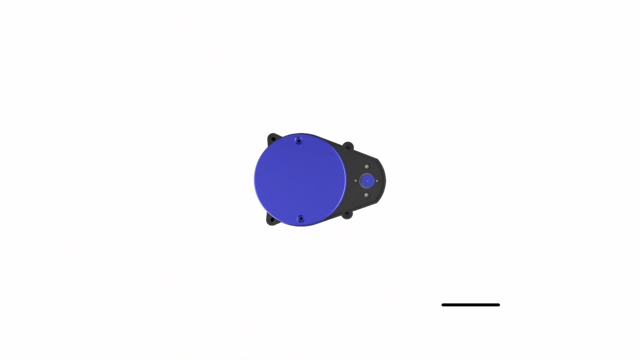 that rotates to get measurements from all 360 degrees. In my case, the lidar can rotate at a speed ranging from 6 to 12 Hz and can read 5000 beams of light per second. So with a simple math we can say that if I use a speed of 7 Hz, I can get approximately 714 points per second. 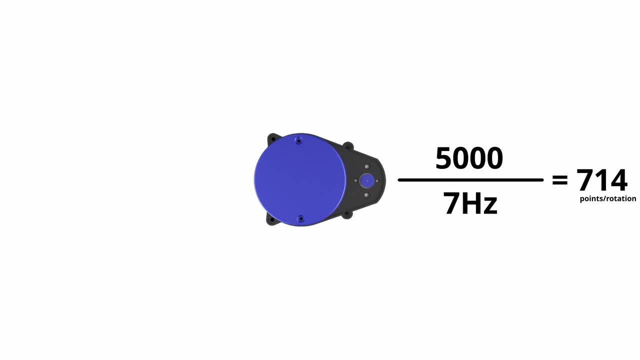 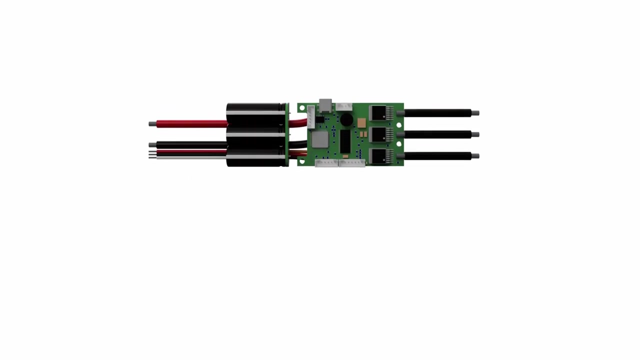 That gives me a resolution around 0.5 degrees. Also, lidars can have a maximum range of distance. Expensive ones can get more than 100 meters, but in my case I can only read up to 10 meters. The VASC is responsible for controlling the brushless motor and also the servo. 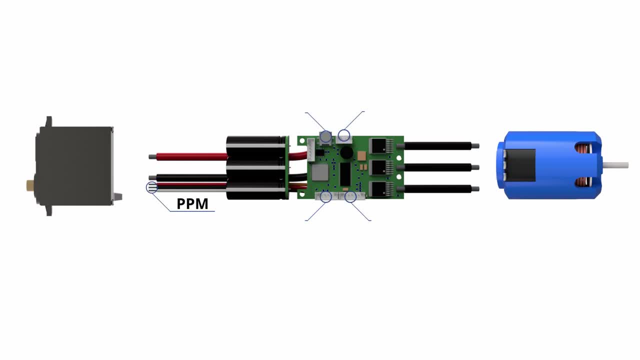 It can interface with PPM signals, UART, I2C, USB and CAN bus. In my case I use USB serial to communicate with the Jetson Nano. I also have the brushless hall effect sensor connected to the board. That gives me a better estimate of the velocity of the car. 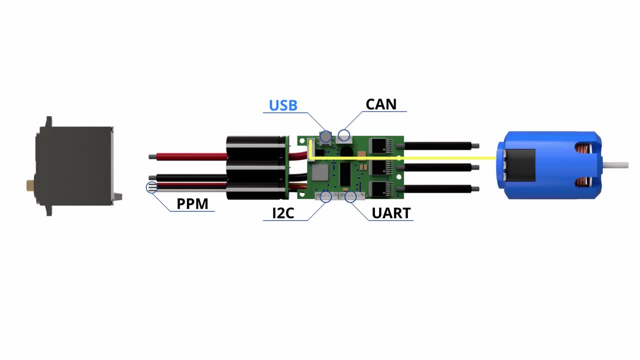 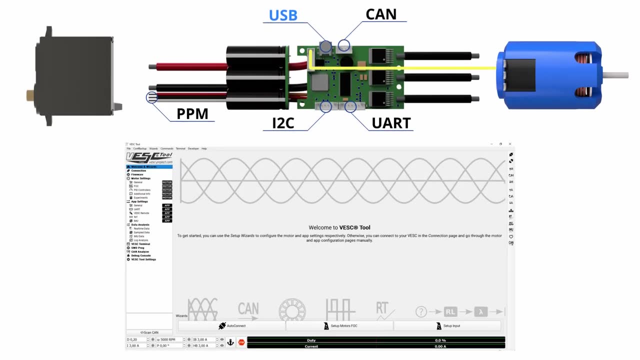 that has an important role in the odometry that I will explain later. The VASC comes with a software that gives you all the freedom to do any type of customization in order to get the best performance of the motor. You can also configure settings for your battery. 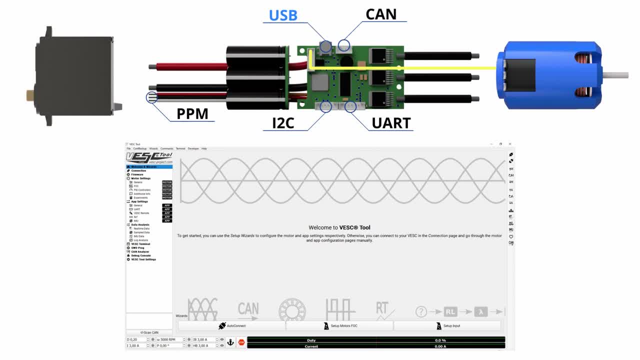 mode of control and inputs used. You can perform autotunes in a very helpful wizard, which is a good start point to configure your motor. Now that I have talked about the sensor and the actuator, we need to join all of this together.